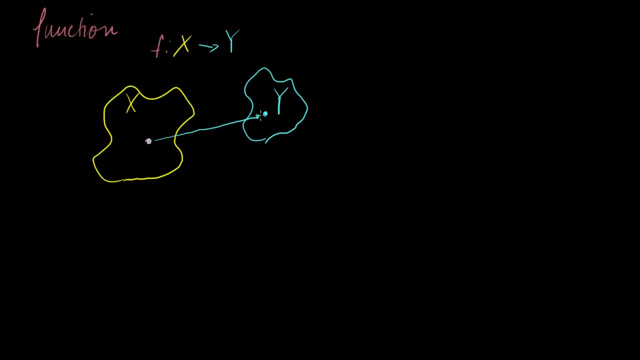 it. I will map it to that member. right there I'll use the word map it, And that really just means relating it to or associating with another member of y. And if you'd give me some other point right here, I'll. 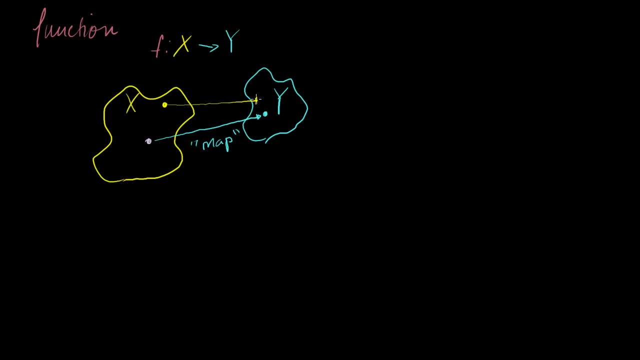 relate it to another member of y. I'll relate it to another member of y right there. I might even relate it to the same member of y, And so this notation just says: this is a mapping from one set, x- and I'm speaking in very general terms- to another set. 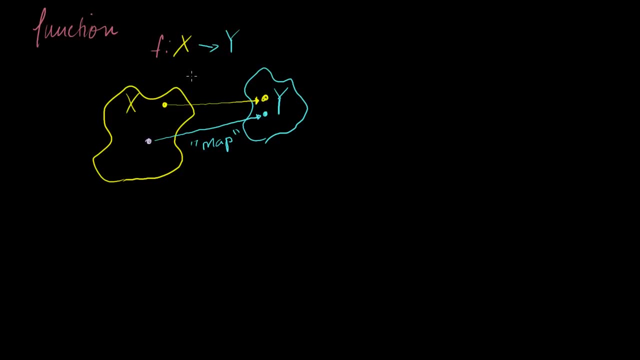 y, And so you're probably saying, hey, Sal, this is very abstract. how does this relate to the functions that I've seen in the past? Well, let me just write down a function. You've probably seen a lot in the past. 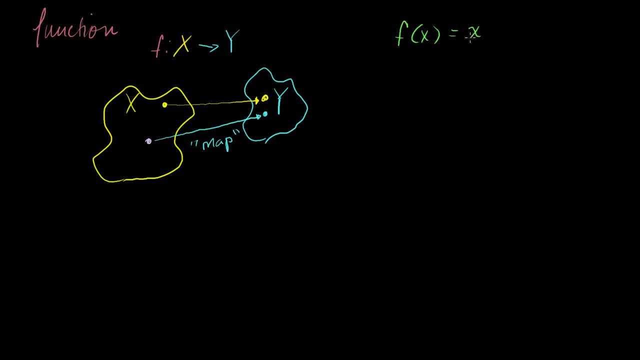 You've seen people write or you've dealt with: f of x is equal to x squared. How would we write this in this notation? Well, this is a function, assuming that it's kind of the traditional way that you see it. this function, 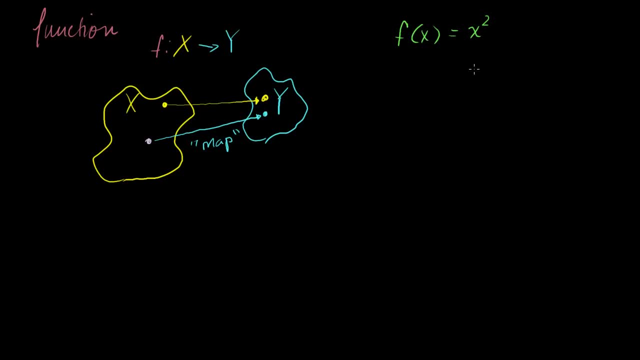 And actually let me just write it with the f. I was going to write it with the g of x, just so that this doesn't always have to be an f, but I think you get that idea In this case: f. 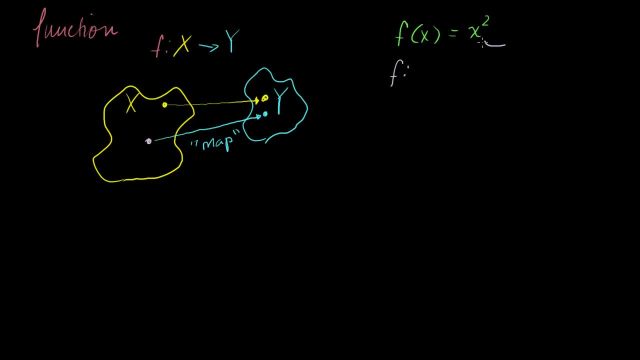 Is a mapping from real numbers, right? The real numbers are everything that I can put in here, And actually this is part of the function definition. I could constrain this to just be integers, or just be even numbers, or just be even integers. 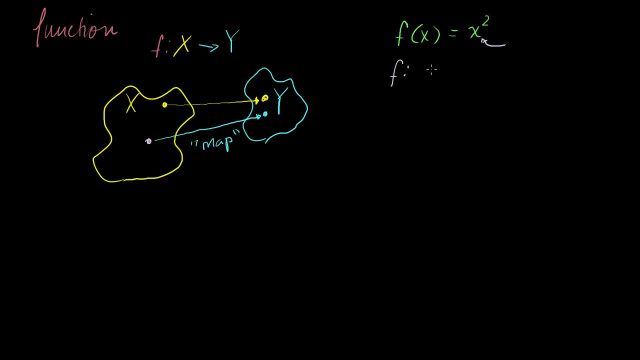 But this is part of the function definition. I'm defining the function to be a mapping from real numbers. I'm saying: you can put any real number here and it's going to map to. well, it's going to map to real numbers. 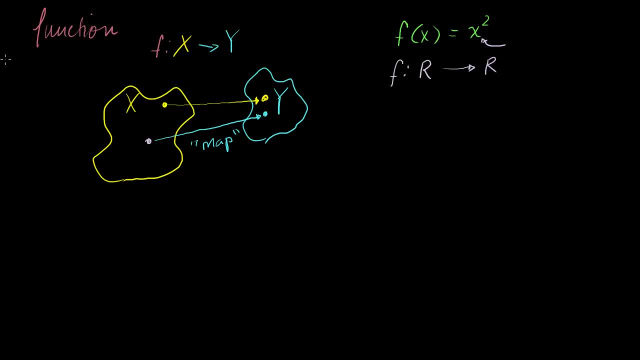 So in this case, if x is real numbers, it's going to map to itself, which is completely legitimate. So if this is the real numbers- and obviously the real numbers would go off in every direction forever- but if this is the real numbers- this function- mapping- is just. 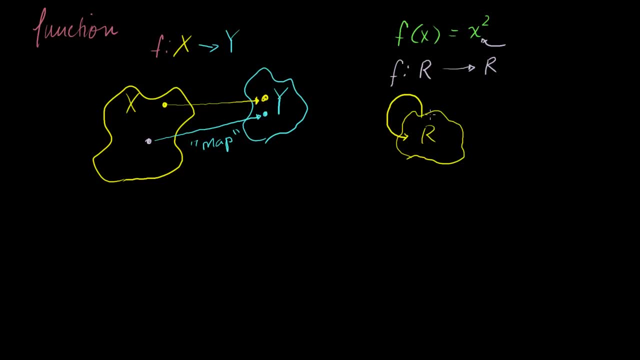 taking every point with f and mapping it to another point, or every point in r and mapping it to another point in r. It's taking every point and associating with it its perfect square. And I want to make a very subtle notation, or at least 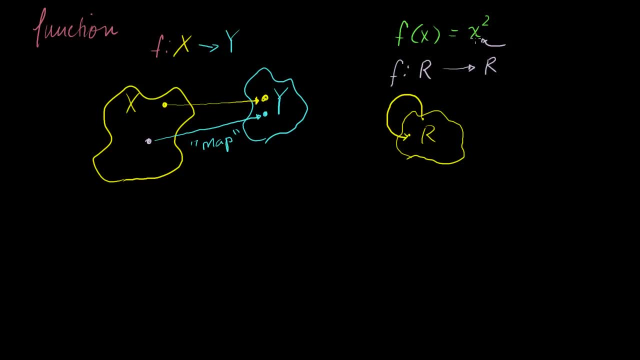 in my mind the first time that I got exposed to functions I was thinking: you give me an x and I square it, and I'm giving you the square of x. And that's true, You are doing that, But at least the way my brain worked, I kind of thought of it. 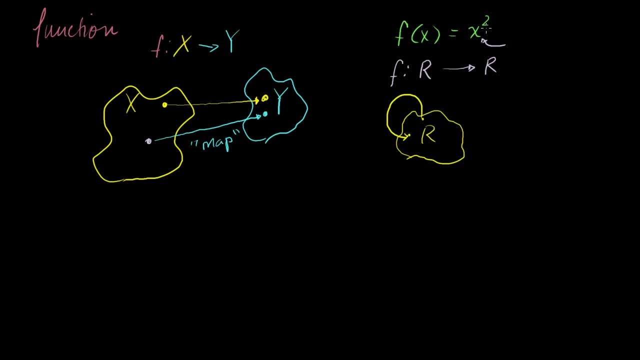 as I was changing my x into another number And you can maybe view it that way and that might actually be the best way to view it, But the mathematical definition I'm introducing here is more that I'm associating x with x squared. 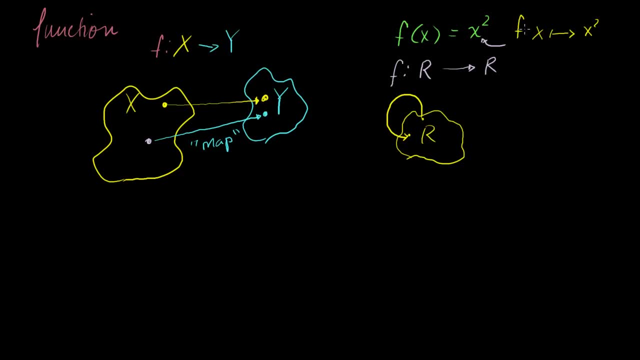 And this is actually another way. This is another function. This is a function notation of writing this exact same thing, These two statements right here. this statement and this statement are identical. This statement you've probably never seen before, but I kind. 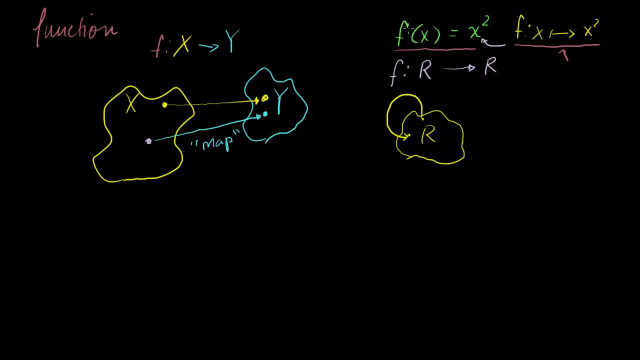 of like it because it kind of shows the mapping or the association more, While this association- I kind of think that, look, you're putting an x into a little meat grinder or some machine that's going to turn, that's going to ground up the x or square the x. 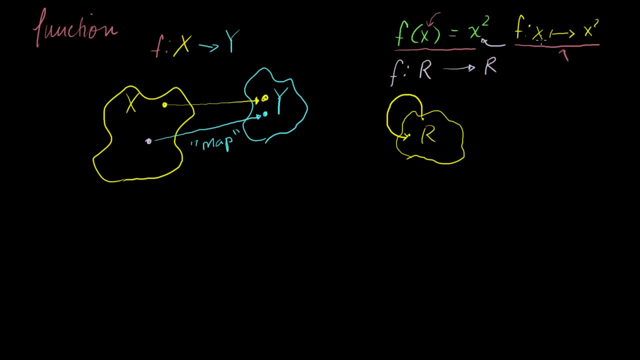 or do whatever it needs to do to the x. This notation to me implies the exact same thing. This is the actual mapping: You give me an x and then I'm going to associate another number in real numbers, called x squared. 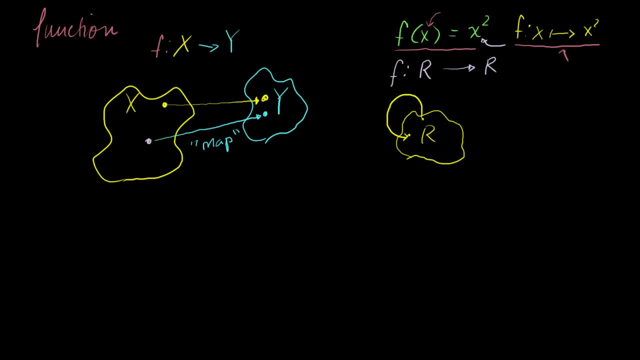 So it's going to be just another point And just as a little bit of terminology- and I think you've seen this terminology before- the set that you are mapping from is called the domain And it's part of the function definition. I, as the function creator, have to tell you that look. 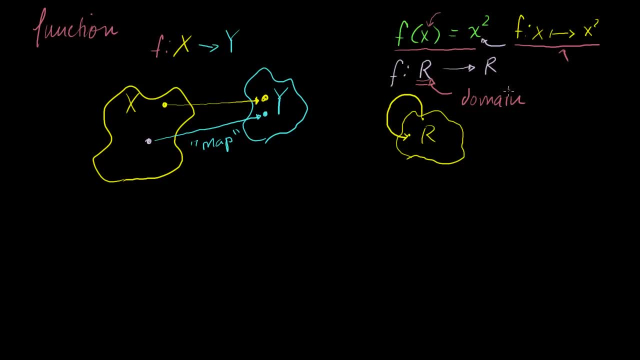 every valid input here has to be a set of real numbers. Now, The set that I'm mapping to this is called the co-domain, And I guess the obvious question that you're probably asking is: hey, Sal, when I learned all of this function? 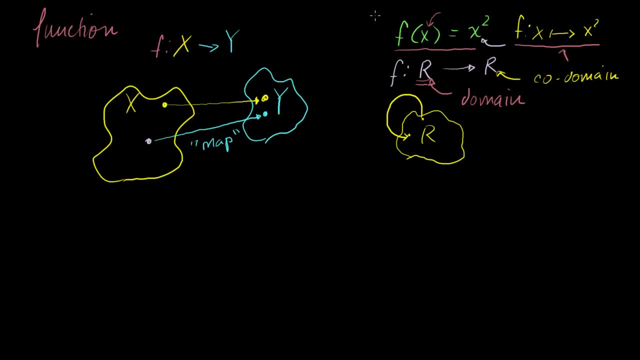 stuff in Algebra 2 or whenever you first learned it. you're like we never use this co-domain word- And actually I don't think it has a hyphen in it- But we never use that co-domain word. We have this idea of range. 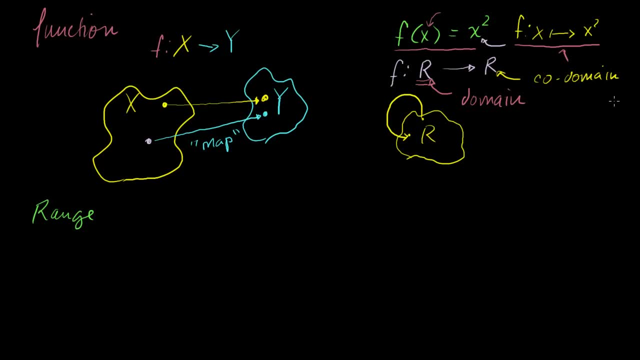 I learned the word range When I was in 9th or 10th grade. How does this co-domain relate to range And it's a very subtle notation. So the co-domain is the set that you're mapping to In this example. this is the co-domain. 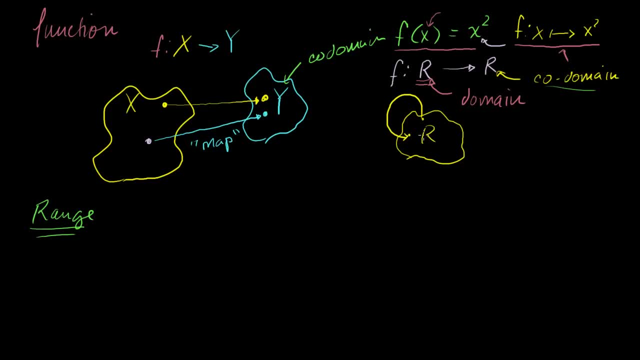 In this example, the real numbers are the domain and the co-domain. So the question is: how does the range relate to this? So the co-domain is the set that can be possibly mapped to. You're not necessarily mapping to every point in the co-domain. 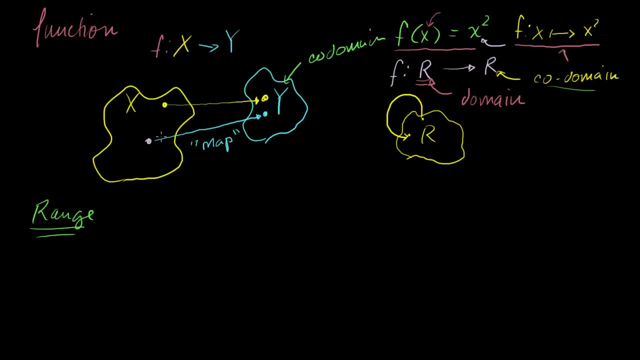 I'm just saying that this function is generally mapping from members of this set to that set. The range is the subset. Let me write it this way. It could be equal to the co-domain. It's some subset. A set is a subset of itself. 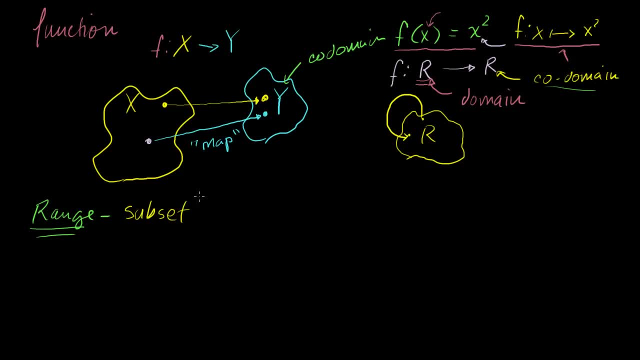 Every member of a set is also a member of itself, So it's a subset of itself. So range is a subset of the co-domain. I keep adding a hyphen there, Or a dash. A dash is a subset of the co-domain which the function. 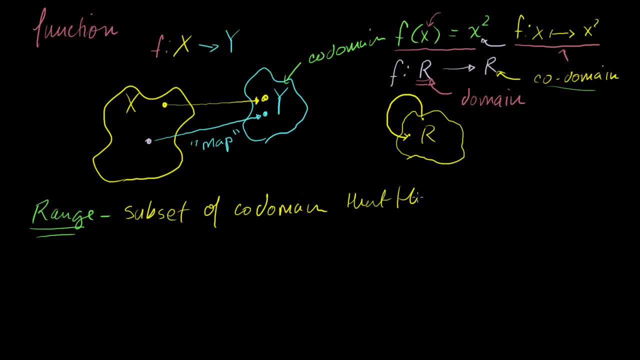 actually maps to. So let me give you an example. Let's say I define the function g And it is a mapping from the set of real numbers. Well, let me say it's a mapping from r2 to r. So I'm essentially taking two tuples and I'm mapping it to. 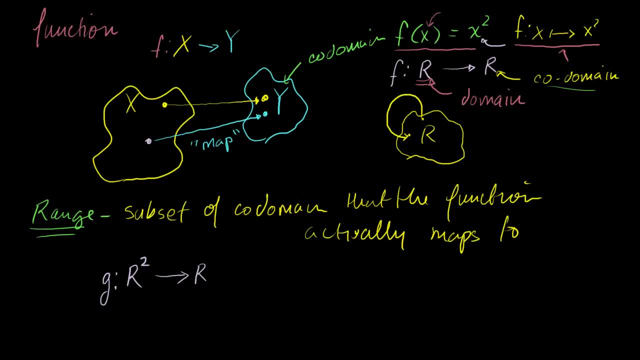 r and I will define g. I'll write it a couple of different ways. So now I'm going to take g of, let's say, two values, So I could say xy, or I could say x1, x2.. 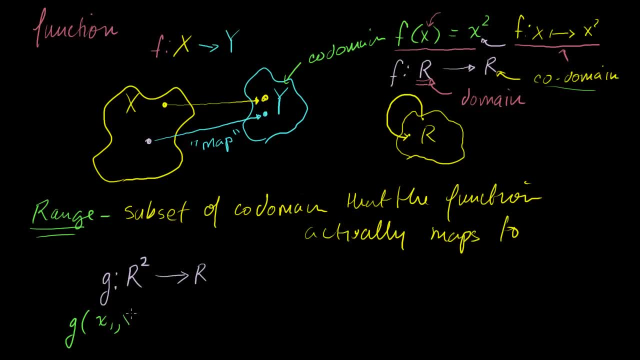 Let me do it that way: g of x1, x2.. Let me do it that way: g of x1, x2.. Well, let's say it's always equal to 2.. It just always equals to 2.. 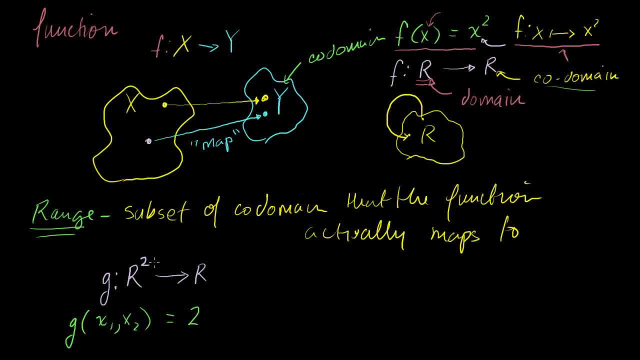 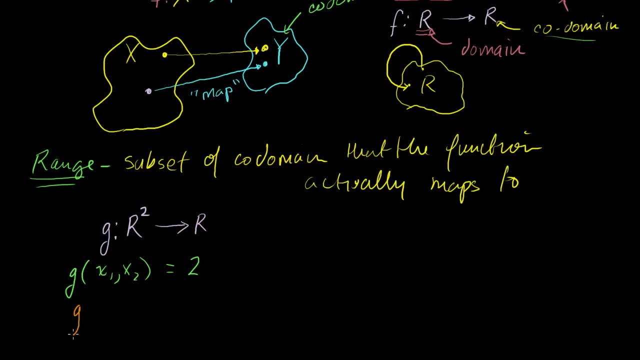 It's a mapping from r2 to r, but this is always equals 2.. So what is our actually? let me write it the other notation, just because you probably haven't seen this much, But I could write g maps any points: x1 and x2 to the point 2.. 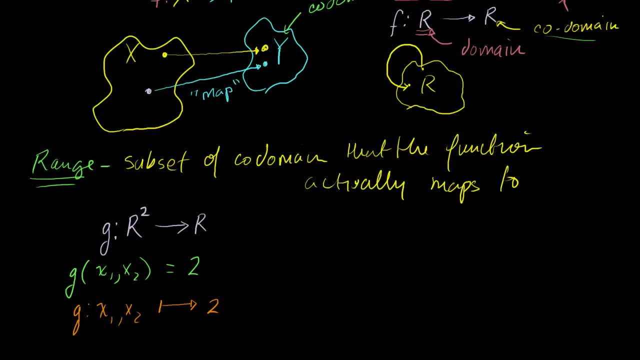 This makes the mapping a little bit clearer. But just to get the notation right: what is our domain? What's the real number? That was part of my function definition. I said we're mapping from r2.. So my domain is r2.. 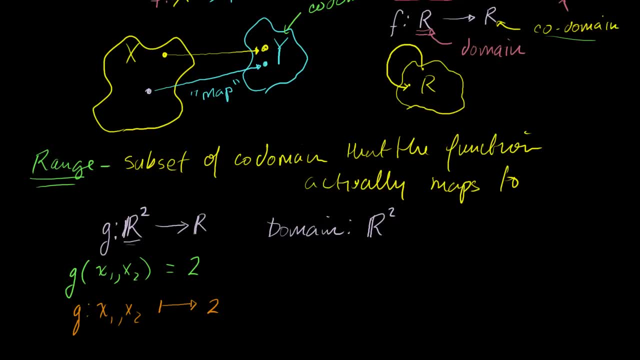 And I should actually make that little line there. Now, what is my codomain? Well, my codomain is the set that I am potentially mapping to, and it's part of the function definition. This, by definition, is the codomain. 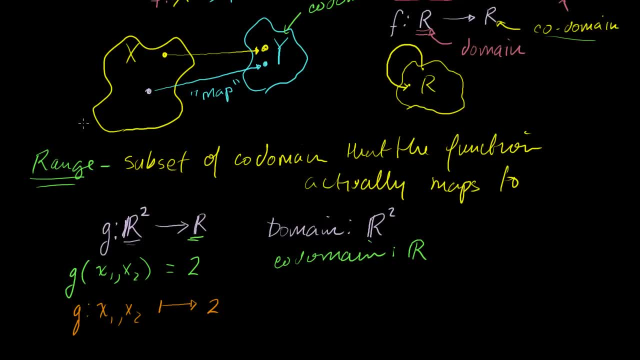 So my codomain is r. Now what is the range of my function? The range is the set of values that the function actually maps to. In this case, we always map to the value 2.. So the range is actually just the value 2.. 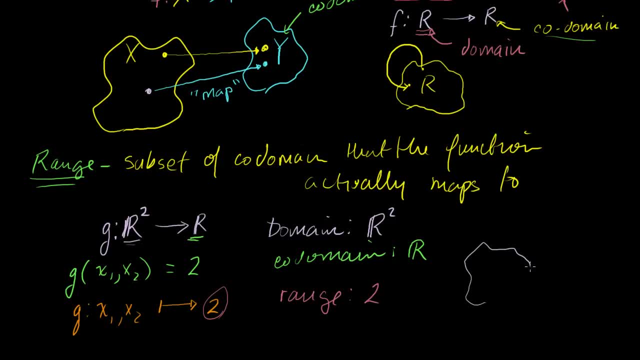 And if we were to visualize this, r2 is actually I wouldn't draw it as a blurb, I would draw it as the entire Cartesian space, but I'm just, I'm just giving you an example. I'm just giving you an example. 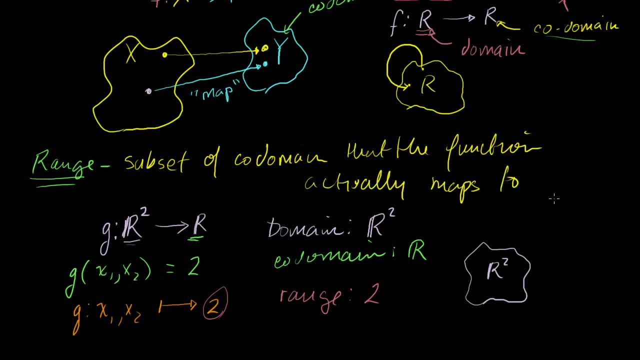 I'm just giving you kind of an abstract notion. That's r2.. If I really had to draw it r, I would draw it as some type of a number line. Actually, let me do it that way just for fun. You don't normally see it written that way. 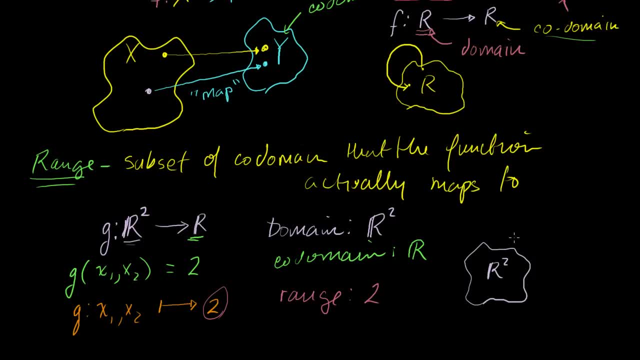 But I could just draw r like that's r2.. And I could just draw r as some straight line. So this is the set r. I could draw it like that as well, But let's just say it's the set r. 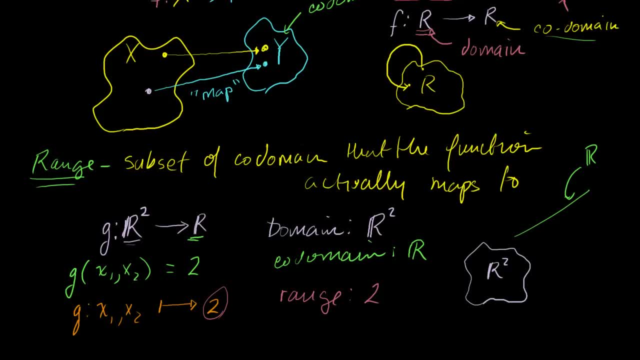 And my function g essentially maps any point over here to exactly the point 2, right. 2 is just one little point in r. My function g takes any point in r2, any coordinate, this is some point. this could be the point 3 minus 5, whatever it. 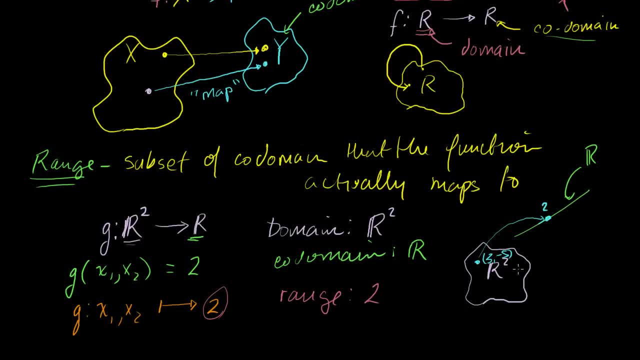 is and it maps it. it always maps it to the point 2 in r. So if I take that point, it maps it to the point 2.. That's what g always does. So g's codomain, you could say it's all of the real numbers. 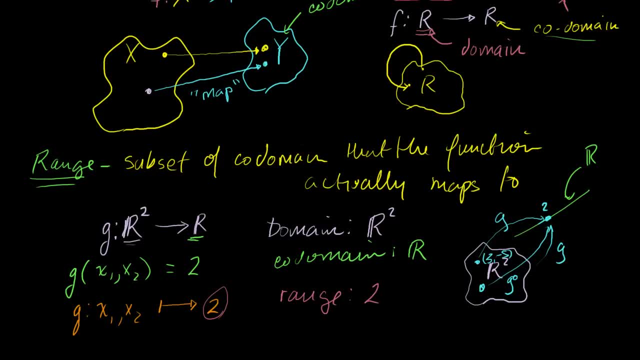 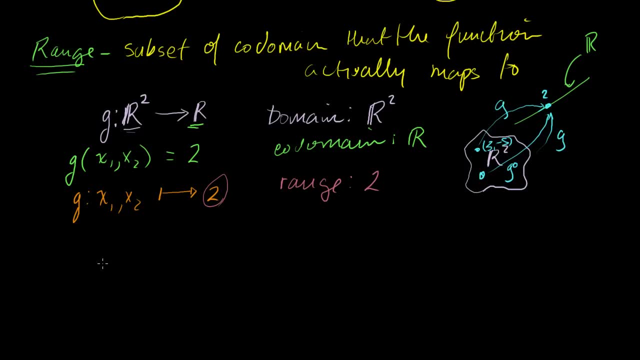 but its range is really just 2.. Now, if I write the example, if I say that let me do another example that might be interesting. If I just write: h is a function that goes from, let's just say it goes from r2 to r3.. 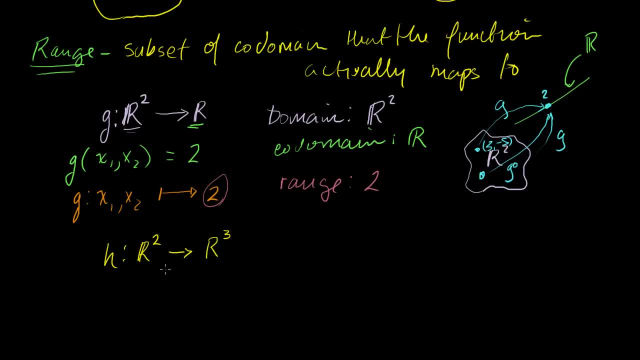 And I'll be a little careful here. h goes from r2 to r3. And I'll write, and I'll write here that h of r2 to r3 is the function g. Now if I write the example, if I say that let me do another. 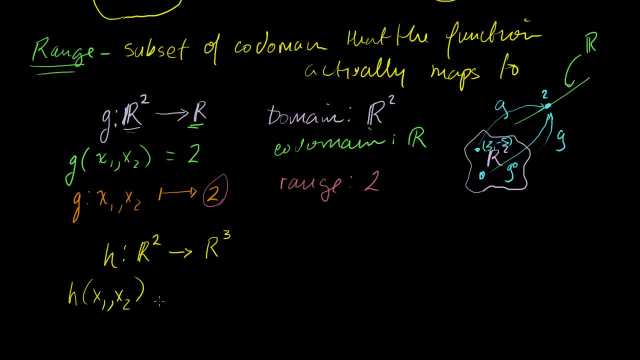 example that might be interesting- x1, x2 is equal to. so now I'm mapping, I'm going to a higher dimension space, so I'm going to say that that is going to be equal to, let's say, my first coordinate. I could say in R3, or my first component in R3 is x1 plus x2.. 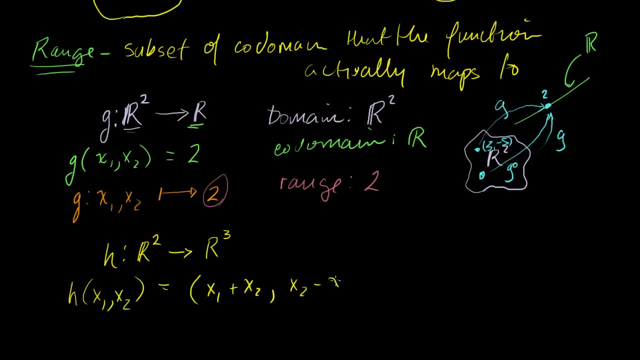 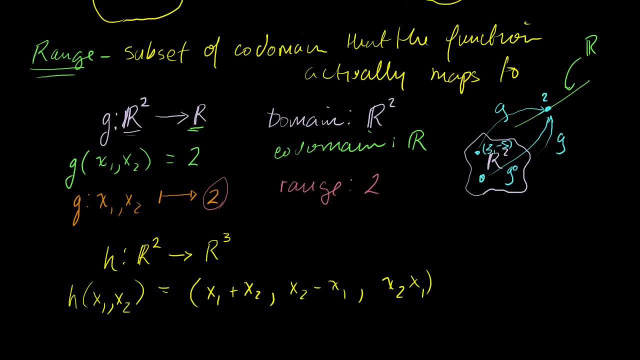 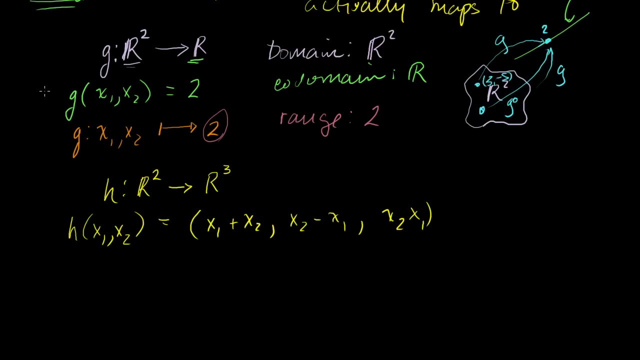 Let's say my second coordinate is x2 minus x1, and let's say my third coordinate is x2 times x1.. Now what is my domain and my range and my co-domain? so my domain by definition, my domain by definition, is this right there? 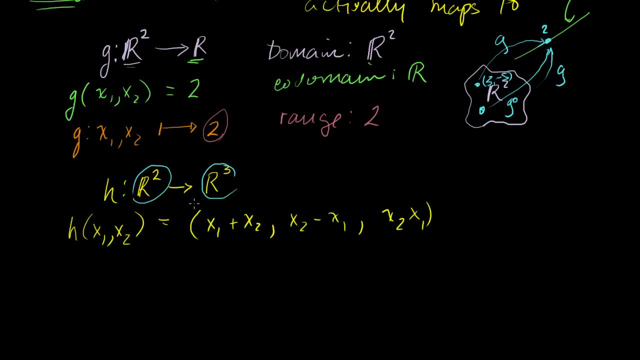 My co-domain, by definition, is R3, and notice, I'm going from a space that has two dimensions to a space that has three dimensions or three components, but I can always associate some point within x1, x2 with some point in my R3 there. 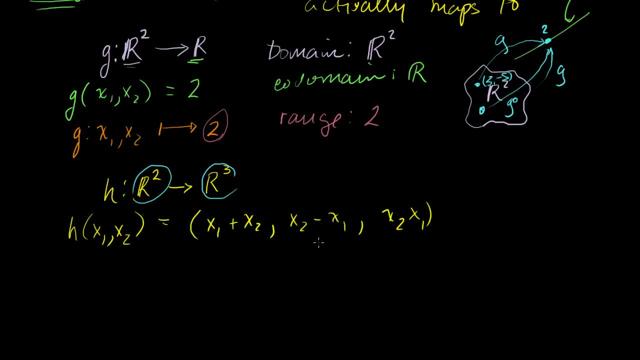 And now a slightly different thing, A slightly trickier question here is: what is the range? Can I always associate every point, every point? maybe this wasn't the best example because it's not simple enough, but can I associate every point in R3, can every point in R3,? so this is my co-domain. my domain was R2,. 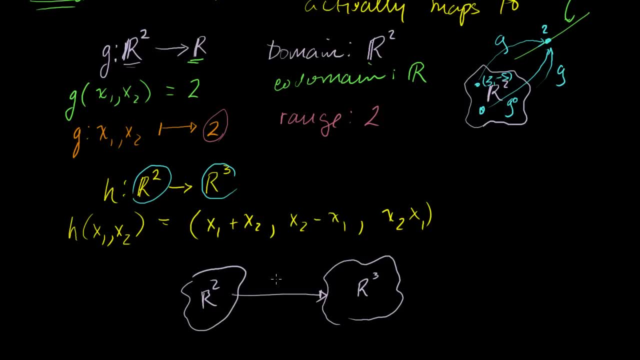 now, and my function goes from R2 to R3, so that's h and so my range. as you could see, it's not like every coordinate you can express as in this way in some way. Let me give you an example. 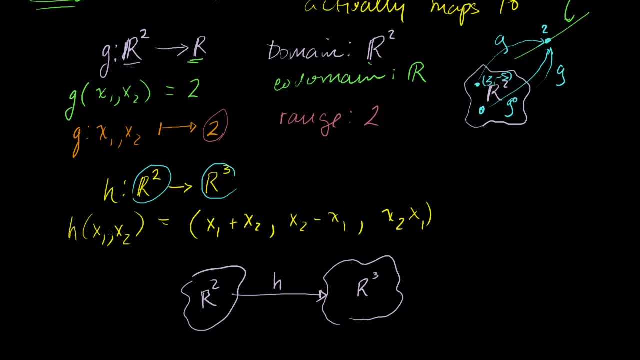 For example, clearly the term. I mean I could put some x1s and x2s here and figure it out. Let's do that. Let's take our h of and let me use my other notation. Let's say that I said h and I wanted to find the mapping from the point in R2.. 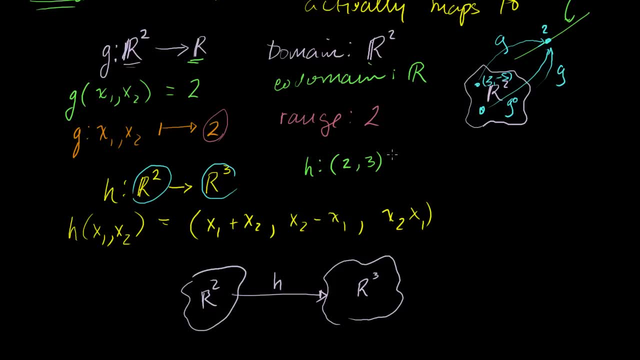 Let's say the point 2 comma 3, and then my function tells me that this will map to the point in R3. This will map to I add the two terms, so 2 plus 3, so it's 5.. 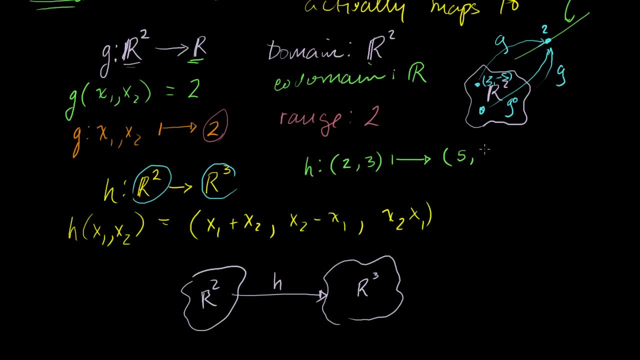 I find the difference between x2 and x1,, so 3 minus 2 is 1, and then I multiply the two 6.. So clearly this will be in the range. This is a member of the range. I shouldn't write it like that. 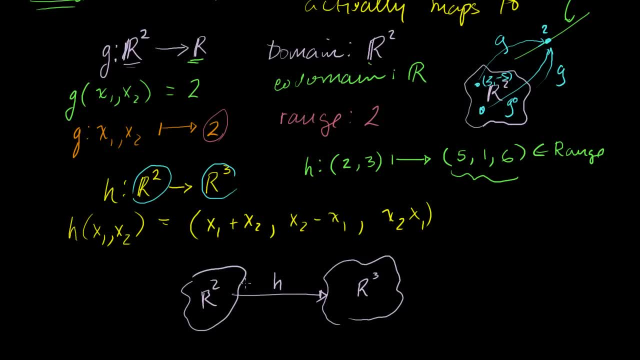 I should write it like this: the member of the range. So, for example, the point 2, 3,, which might be right there, will be mapped to the three-dimensional point. It's kind of just drawn as a two-dimensional blurb right there, but I think you get the idea. 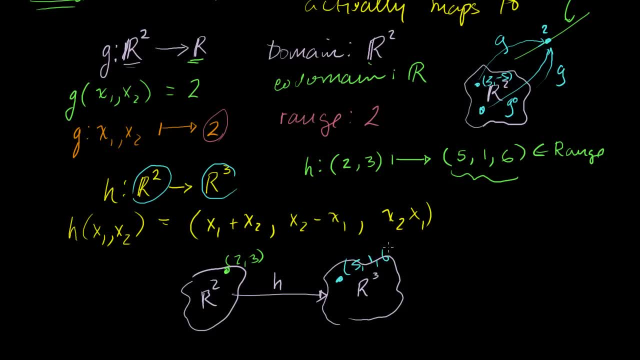 It would be mapped to the three-dimensional point 5, 1, 6.. So this is definitely a member of the range. Now my question to you: if I have some point in R3, let's say I have the point. 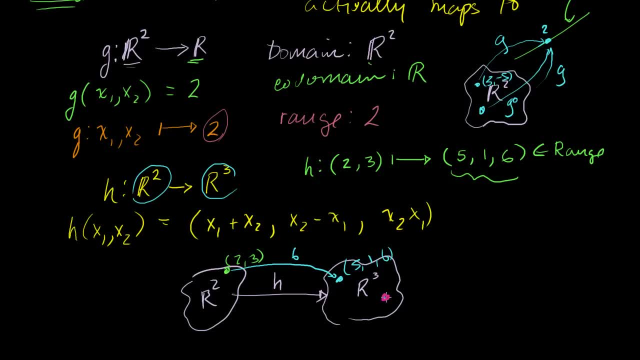 let me do it in a different color. Let me say I have the point. Let's say this is the point 5, 1, 0.. Is this point a member of the range? It's definitely a member of the codomain. 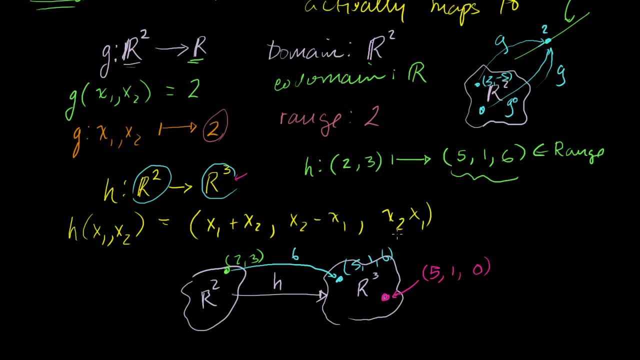 It's in R3.. It's definitely in here and this, by definition, is the codomain. But is this in our range? Well, 5 has to be the sum of two numbers. The 1 has to be the difference of two numbers. 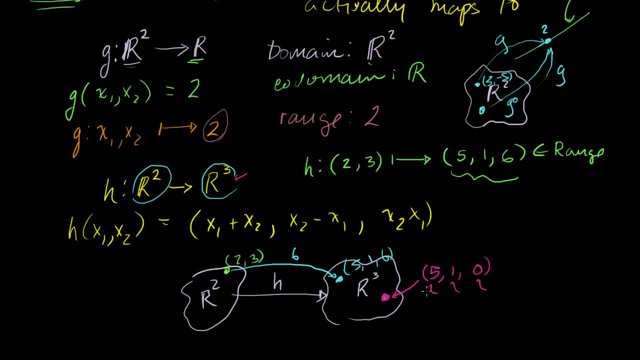 And then the 0 would have to be the product of two numbers And clearly we know 5 is the sum and 1 is the difference. We're dealing with 2 and 3. And there's no way that you can get the product of those numbers to be equal to 0.